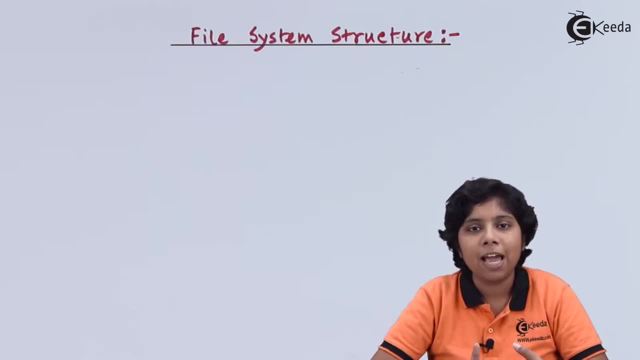 the directory, the files, entry in the mapping and all the directory structure that is maintained in the users directory within it. and the second issue is the translation of the logical address mapping from the physical storage secondary option. now, in this way these two design problems can become the file system structures hindrance. now the file. 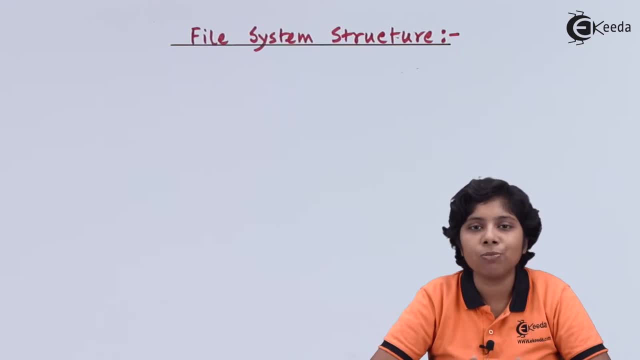 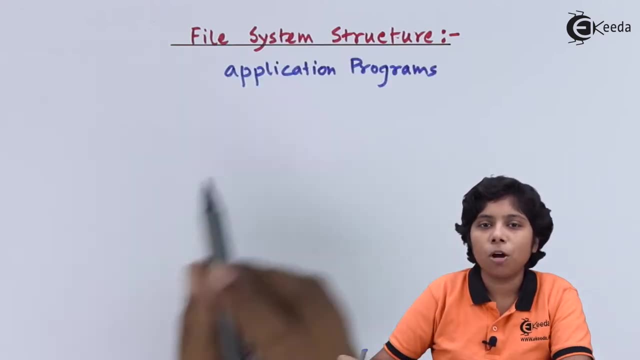 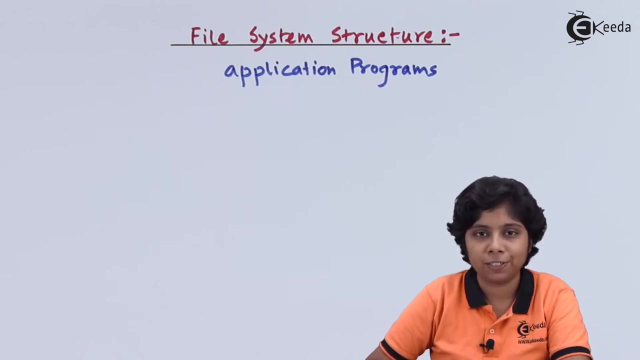 systems optionally uses a layered structure which we will describe in details now. first we will see the layered structures of the file system. at the end. the top of the file system structure is the application programs that are the end products of the results of all the operations now in this file. 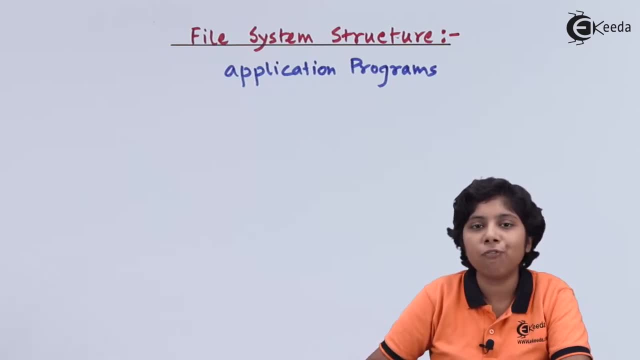 system structure that is made to the user. we should define the attributes of a file, the operations that are to be made to the file and all the directory entry that is mapped from the logical to the physical section. now, from this, application programs, there are almost another layer. 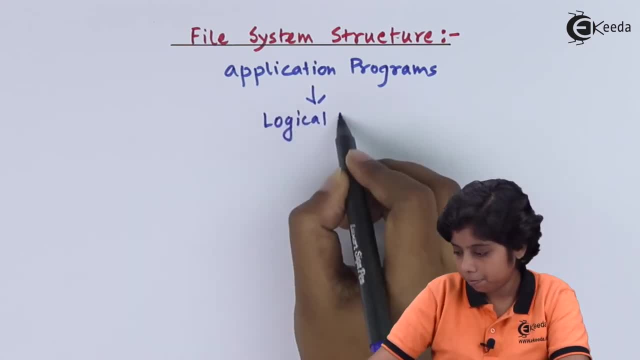 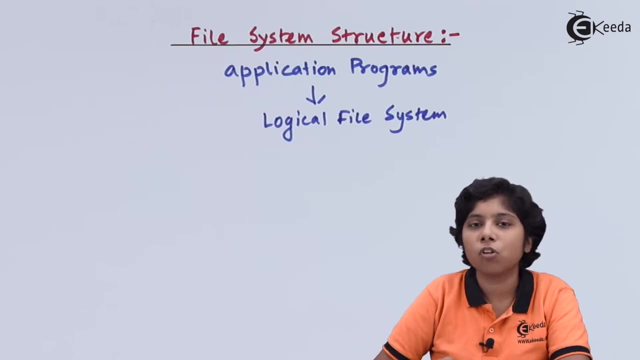 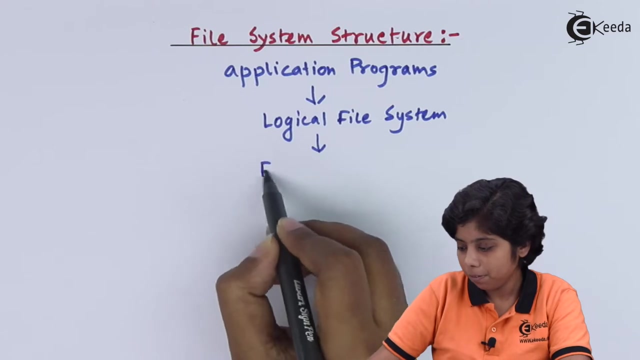 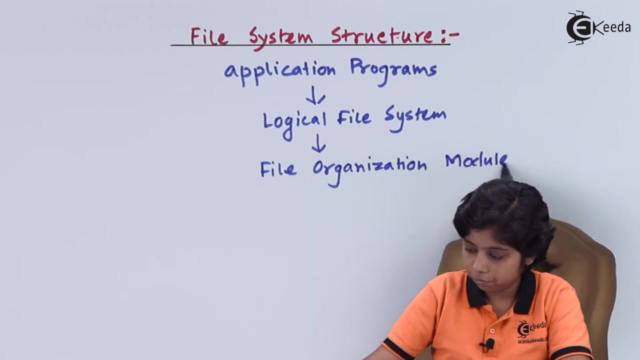 you. the next is the logical file system, which contains a software information about the files. the next is the file organization module, which actually organized the file information control, the translation of the logical to the physical file and with so one basic file system. it not only generates the basic file. 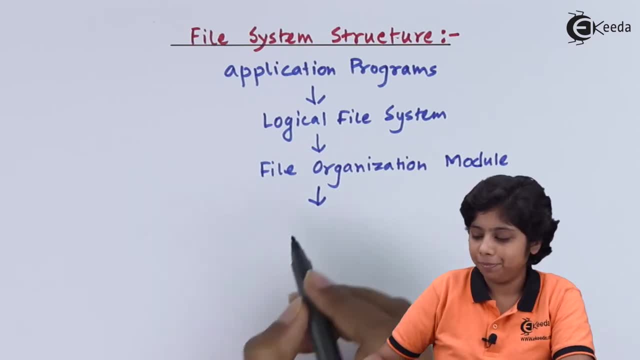 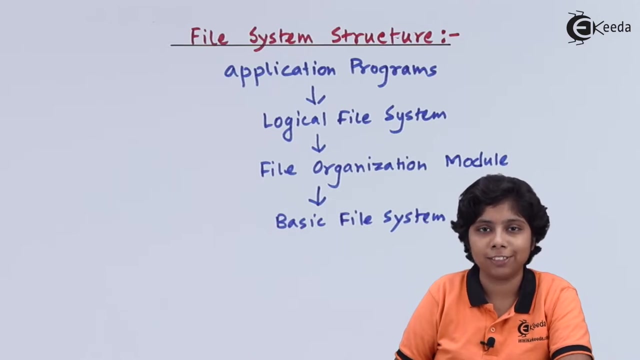 expressions, but also the function day. can Yo applying all these controls? centro N international. the next is the basic file system. this basic file system generally deals with the codes of the output and input of higher level and producing hardware level instructions. the next is the. the next is the comfortable a hundred user access control l and the 적os Pirat. 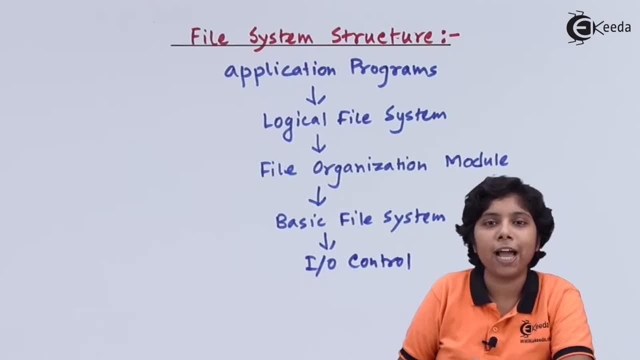 And the last are the devices that should be made and stored on the disk to contain the file information. So here it is moved from the low level to the higher level And each level uses the higher level features can be made up from the low level features. that is configured here. 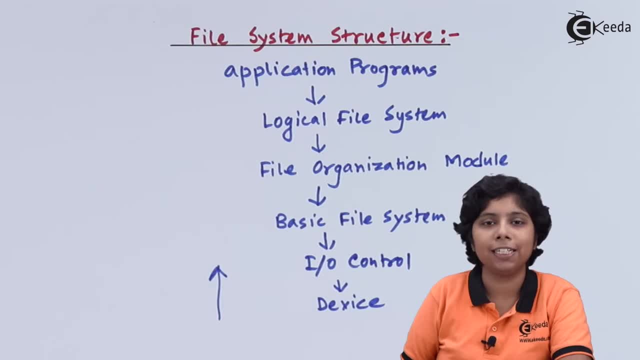 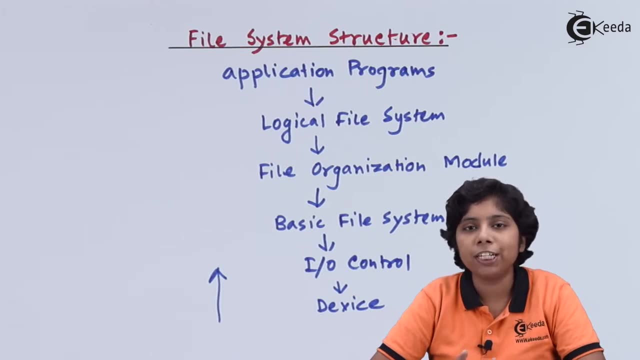 So now we will discuss about each of these layers in details. The IO control level generally consists of the device drivers and the interrupt handlers, which will in turn handles the translation of the logical memory to the physical memory. Now, inputs of this IO controller and the device driver is specifically higher level programming commands like retrieve, block 123.. 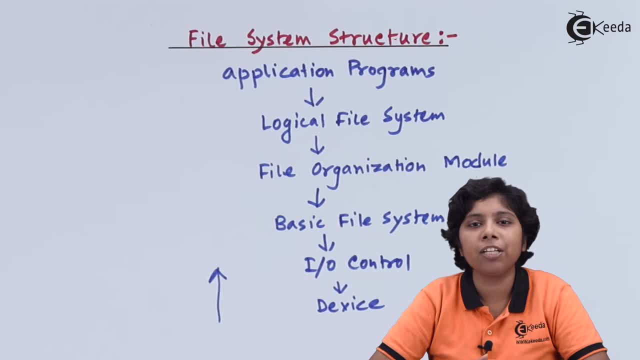 And then we can say that we are having the output as a more lower level, hardware oriented command or outputs Which can be understand by the hardware and then which can be used as a machine level instruction. So in this way the hardware control output can be given as an input of a higher level or the machine level output. 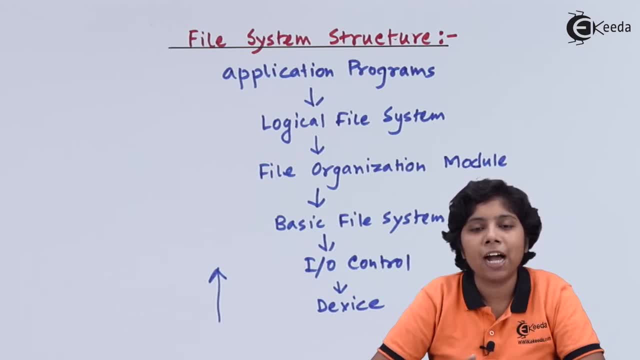 Now this hardware instructions then identify as the IO controller from the rest of the operating system. Now the device driver writes the specific bit patterns to specific locations of the devices To tells us that which device location is to use and what is the action to take place. 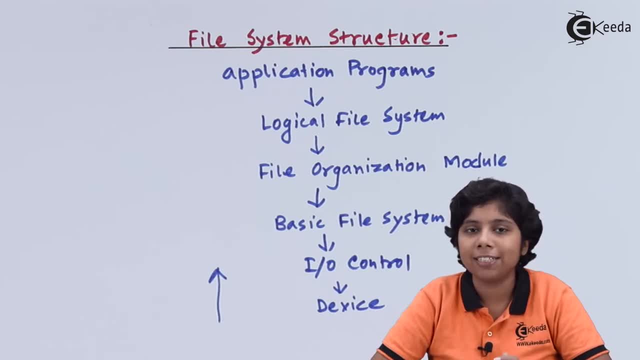 So in this way IO control is done by all the devices using this device structure and then performing the IO control on that particular device: drivers and interrupt handlers, The next. we will move to the basic file system. Now, the basic file system can only issue some generic commands. 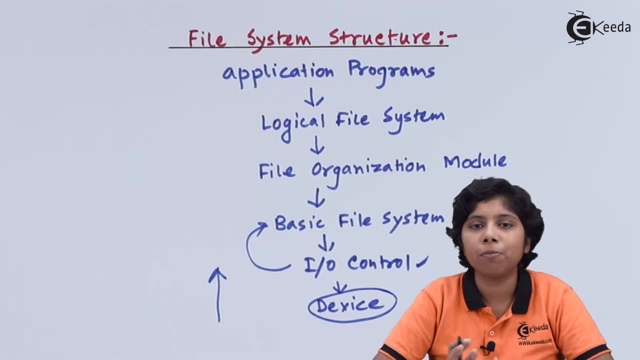 Like from the physical blocks And retrieve data from this physical blocks. Now the physical blocks are identifiable as the integer constant addresses, Like, say, track 2, sector 23,, block 51 and then drive 52. So in this way we can address to the integer values from the physical blocks. 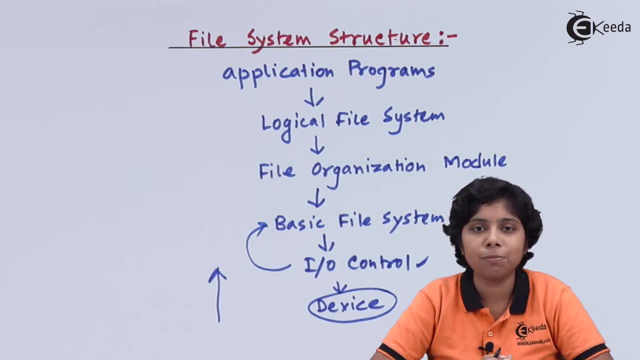 Now this physical blocks are to be mapped to the logical file systems to match the numbers. Now this layer also manages the buffers and the commands. This is your basic focus of the system. This little bit here is for the manager to take a look at the probability of the changes. 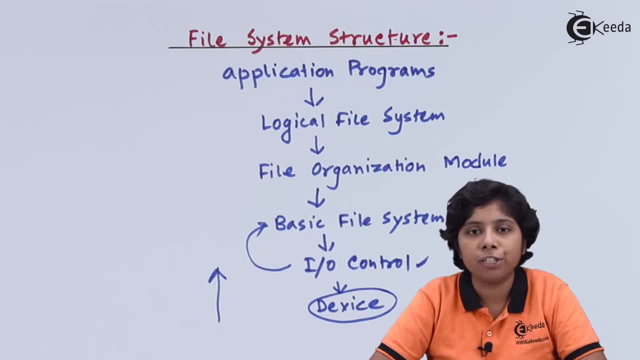 This is for the manager to look up the differences between the block structures. Now the block structures are two block structures. A block is basically a block with two different tiny little an hyphens that are oben on it. These blocks represent the number of memory cell. 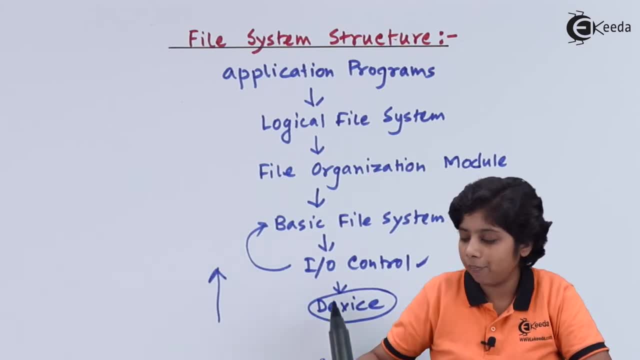 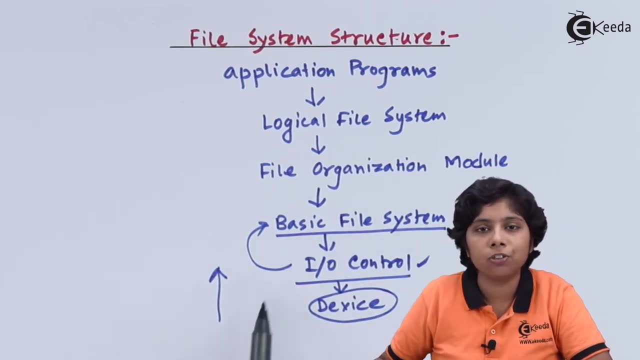 The number of memory cells are 12.. The number of memory cells are four. The number of memory cells are 15.. And these block structures are six. They are called block structures. the basic file system also maintain all the io control and the device information and the metadata. 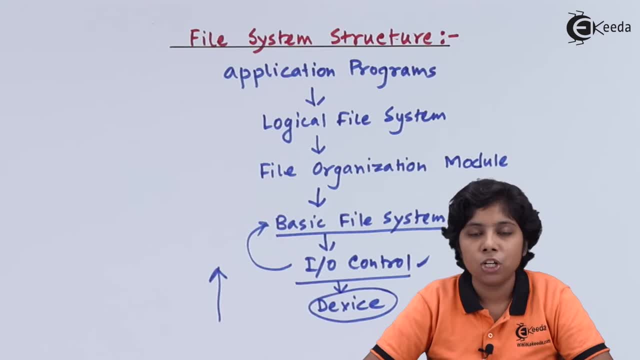 that is the basic constitution of a file system, so its implementation and maintenance is an crucial importance to the file system maintenance. the next layer is the file organization module. file organization module knows about the files, their logical address and their physical address. now, by knowing the type of the file that is to be transferred and the location of the file, we can 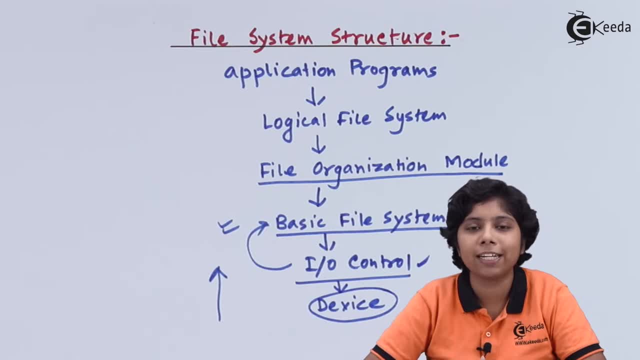 actually translate the logical addresses to the physical secondary storage devices. now the logical addresses can range from, as we have mentioned in the basic file system, say from 0 or 1 through n, but the physical memory space or the addresses of that particular files are different from each other. now there should be a translation from the logical. 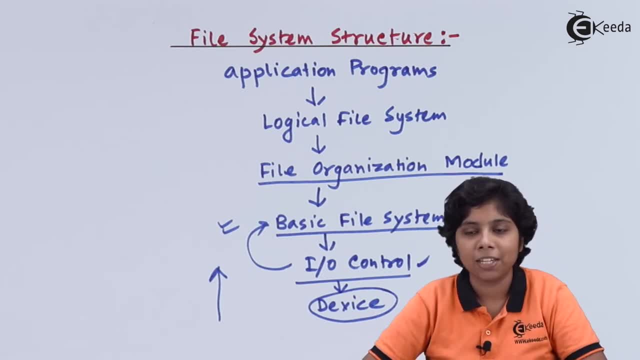 surveillance system to the physical memory space of that primary storage device. now the logical memory space is different from each other. now there should be a translation from the logical file system to the physical system must be done, and this is done by this fargo organization module. along with this translation, it also keeps up an information of the free space manager. 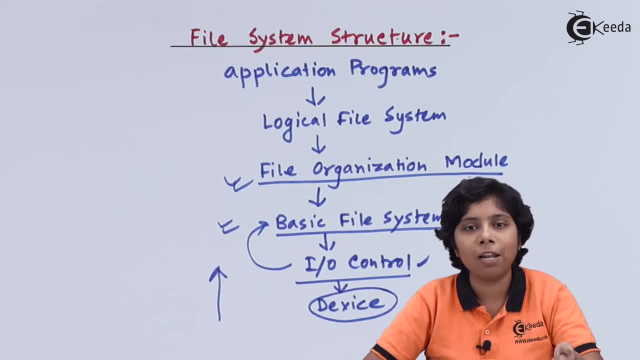 which allocates the unallocated block to the file manager that is to be requested and then needed by the file organization module. so the free space manager then generally collects all the unallocated blocks and then request it on the file organization module. the next step is the logical file system. 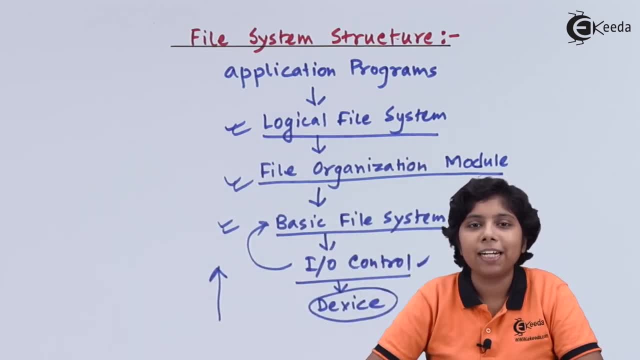 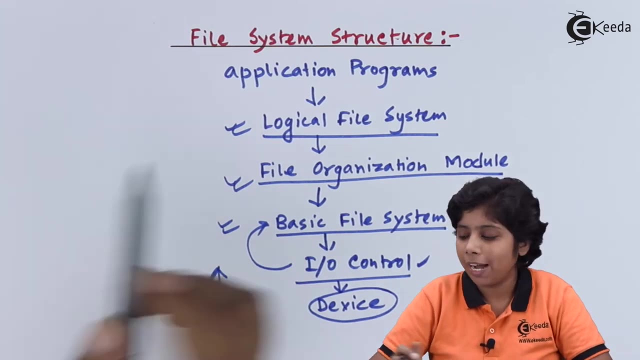 finally, we are reaching this logical file system that is containing the metadata of a particular file system. we know that the metadata constitutes all the file system structure information, excluding the contents or the basic modes of the files. so the files is containing the structure, wise in the logical file system. 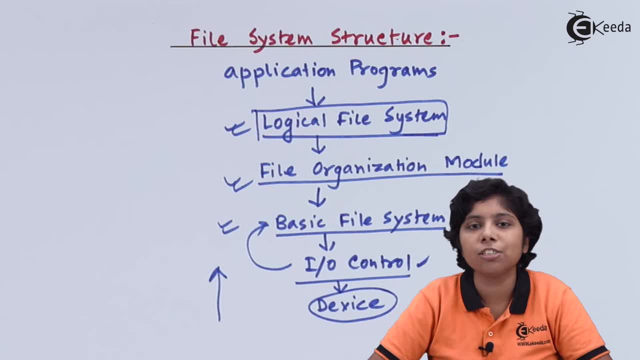 and this logical file system then searches through the directory to maintain the directory structure and to tell us the device driver that what operations is going on that particular device. the file attributes are stored in a file control box and fcb, which is maintained in this logical file system. this fcb contains the file attributes, likes, owner, permission, location of the contents of. 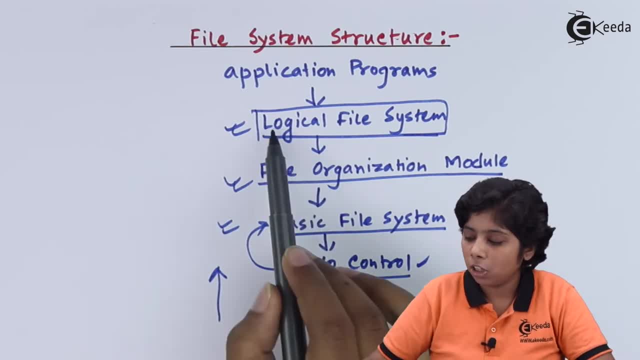 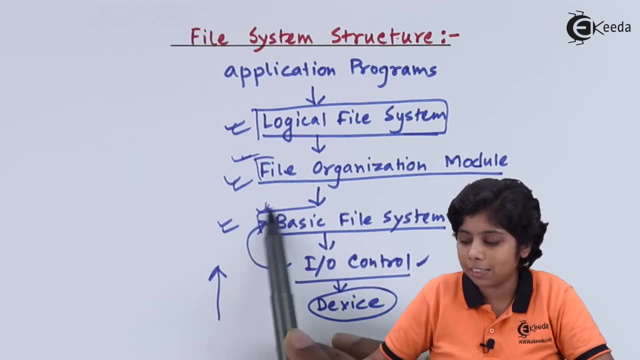 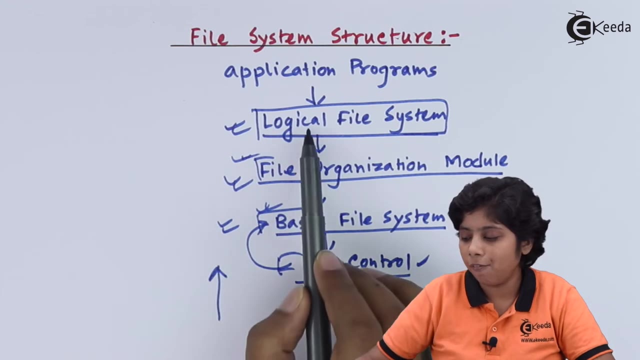 the files and so on. so in this way, the logical file system uses the file organization modules, physical madras mapping, which uses the basic file systems, generic issues, comments, and the io control, which uses the devices so we can see the every layer is, uses its lower level features to use its own features. 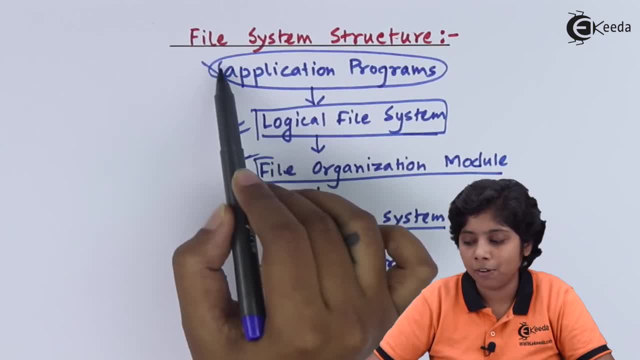 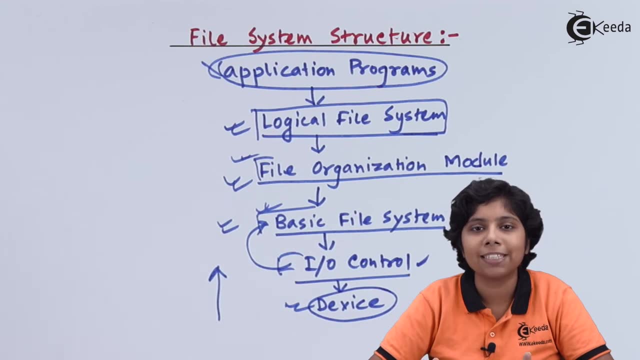 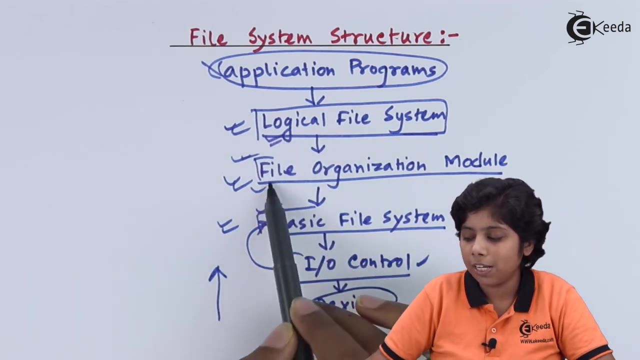 now, as the application programs or the end product is are given to us, then we can say that this layered architecture can allow us to use multiple file systems in a single system. so a file system can use can have more than one logical file system and file organization modules within it and a transfer of data between these organization. 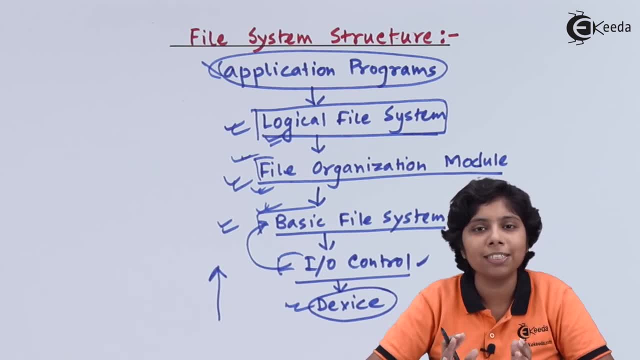 modules and the io control blocks can takes place very seamlessly, like an unix file system or ufx, which is based on the berkeley first file system, or bffs, also produced by the microsoft windows of windows operating system, like fat, fat32, andwnpfs, that is, a windows community file. 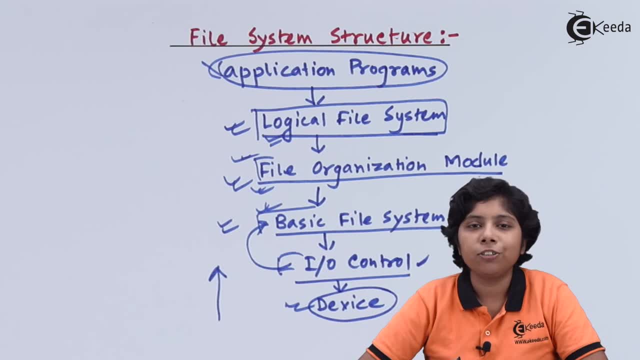 system is also used in this many types of different file systems. it also uses cd-rom and dbd-rom or dvd-rw file system structures. although linux uses over 40 types of multiple file systems in, the standard solution of a file system in linux is the generally extended file systems. 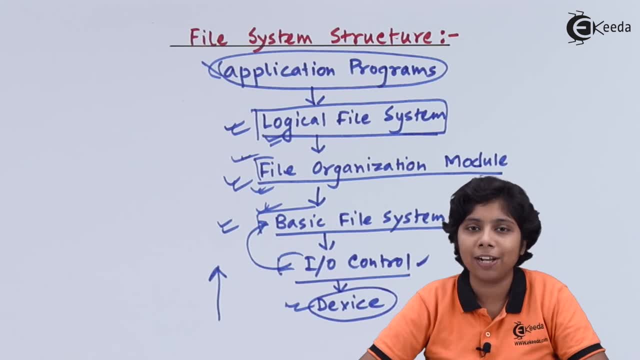 as ext3 and ext4 versions of the linux file system to use now for the layered architecture is very implemented easily and seamlessly, but there are also overhead of designing the operating system. now the operating system designer needs to take care of how many layers should be. there should. 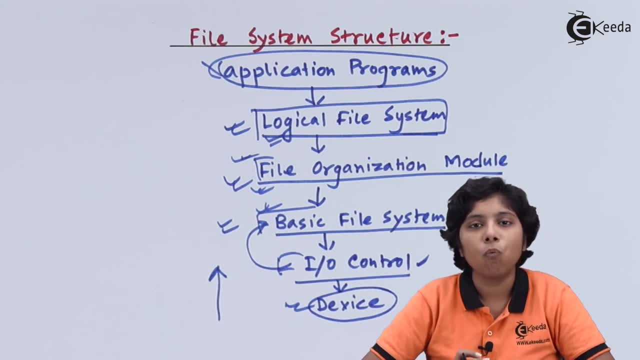 be there in the file system structure and then what layer should perform what operations. so this should be done in the operating system design level. so that is why layered file system structure is often seldomly adopted and then used. now the distributed file system, which is another type of file system, that is, an application program, uses different